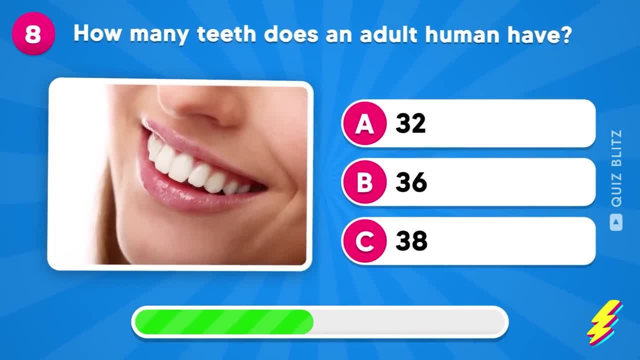 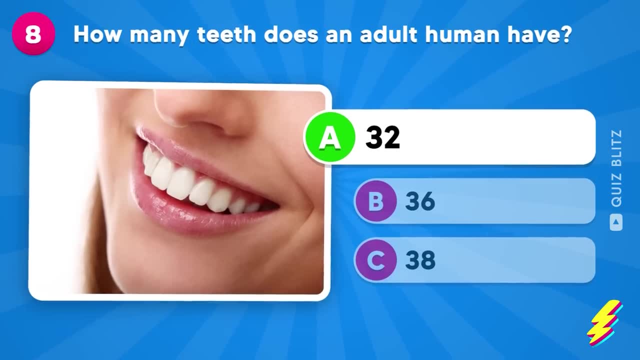 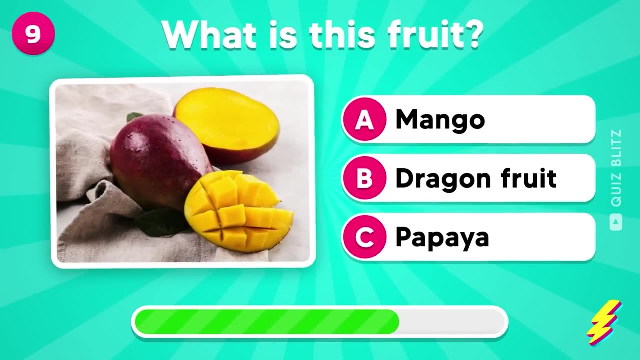 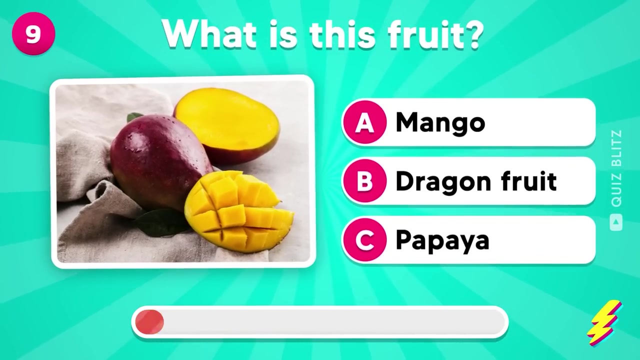 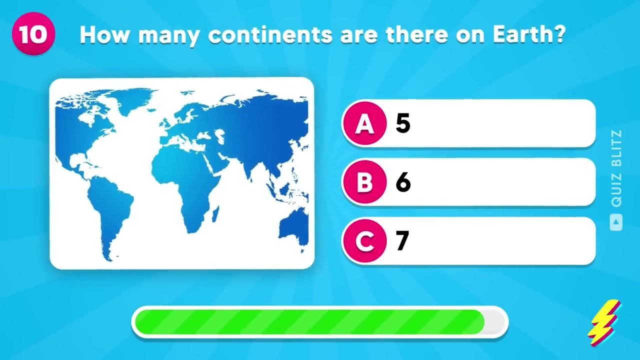 32,, 36, or 38?? Yes, it's 32!. Yes, it's 32!. What is this fruit? Mango, dragon fruit or papaya Mango? How many continents are there on Earth? 5,, 6, or 7?? 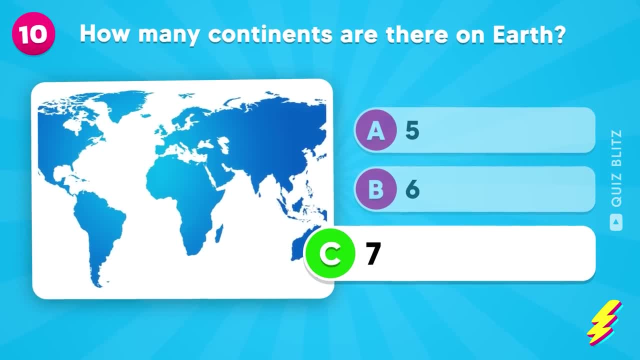 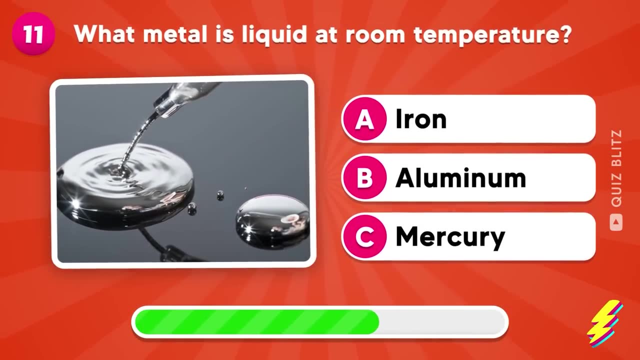 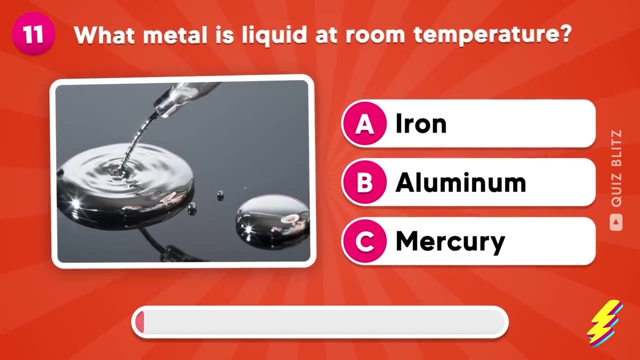 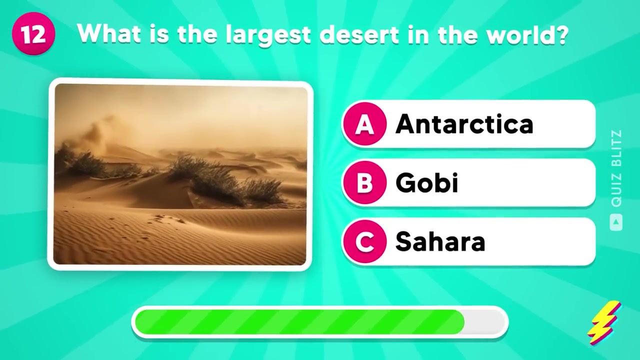 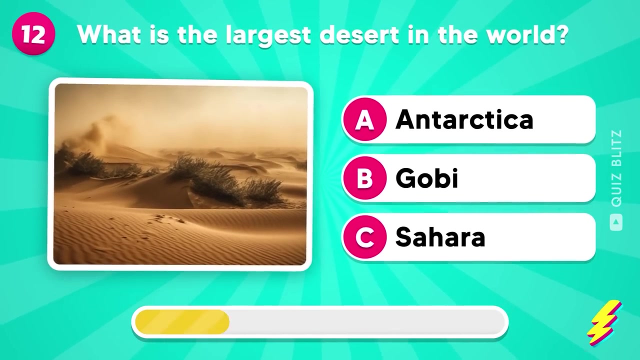 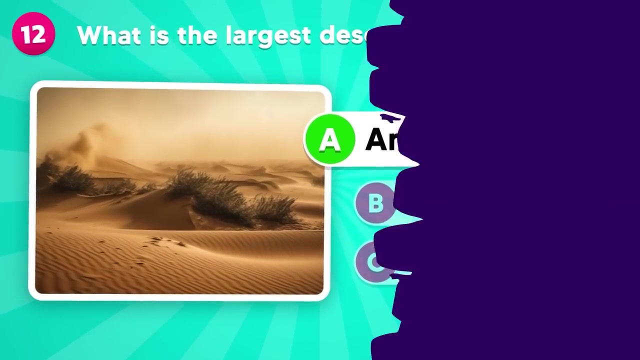 7. What metal is liquid at room temperature? Iron, aluminum or mercury, Mercury? What is the largest desert in the world? Antarctica, Gobi or Sahara? Antarctica? Which chess piece can only move diagonally? The bishop, the king or the rook? 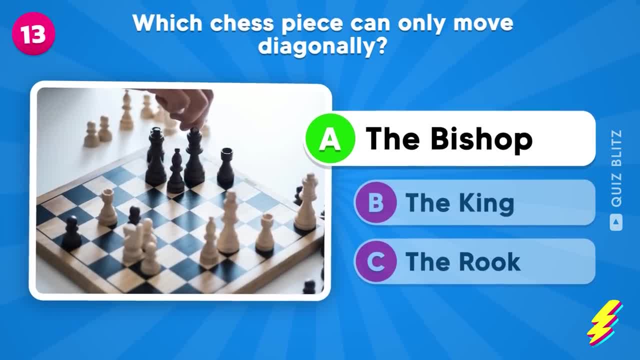 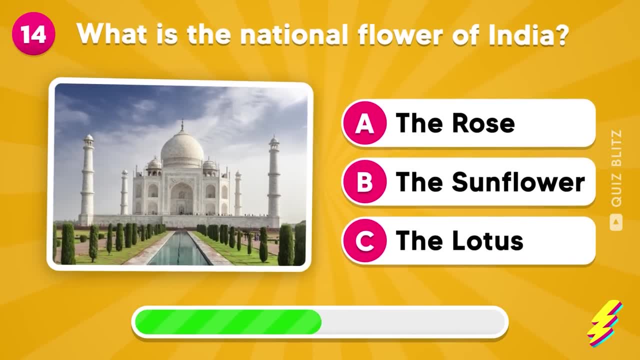 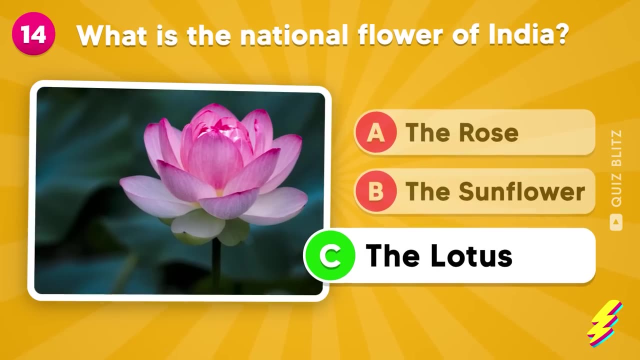 Correct, It's the bishop. What is the national flower of India? The rose the sunflower, or the rose The sunflower Or the lotus? Yes, It's the lotus. Which country has the highest population in the world? 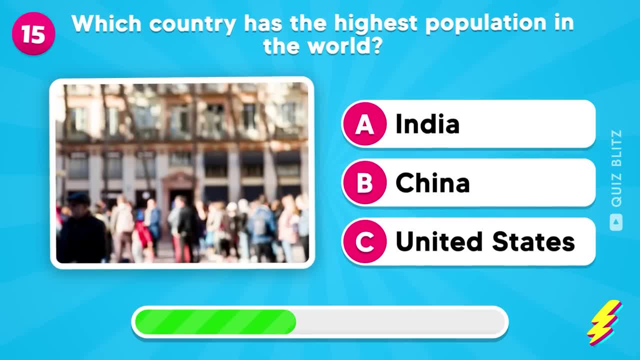 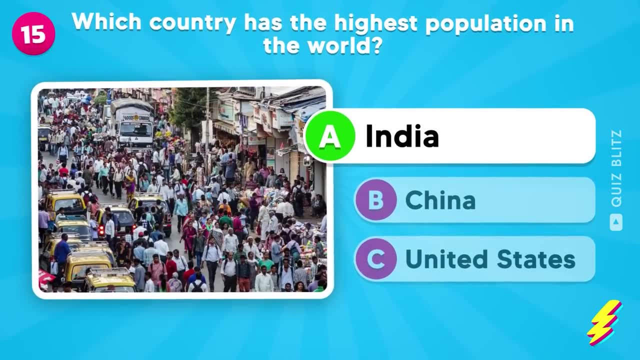 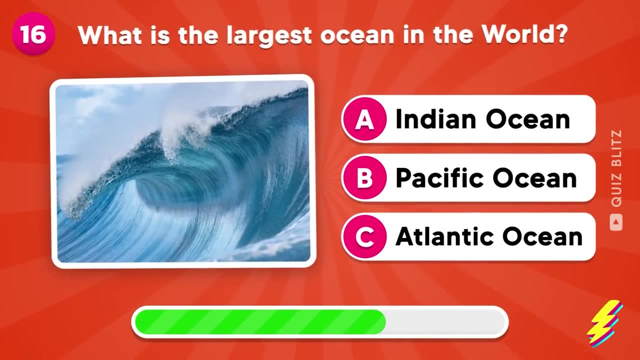 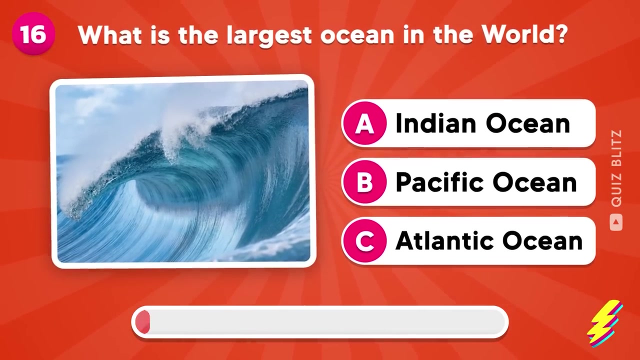 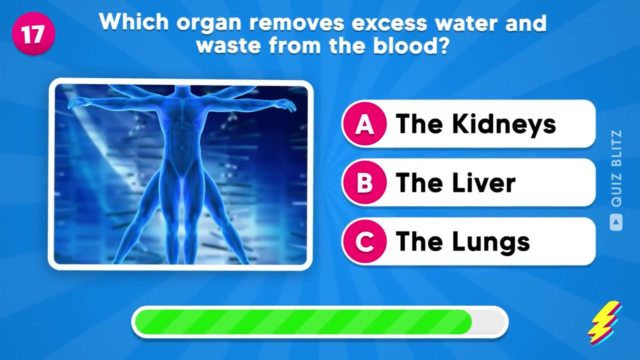 India, China or United States? It's India, with over 1.4 billion inhabitants. What is the largest ocean? Indian Ocean, Pacific Ocean or Atlantic Ocean? Bravo, It's Pacific Ocean. Which organ removes excess water and waste from the blood? 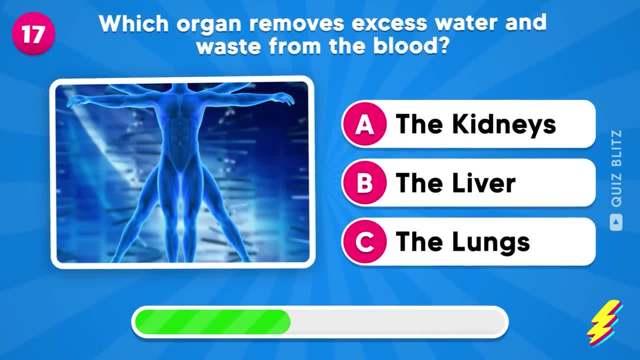 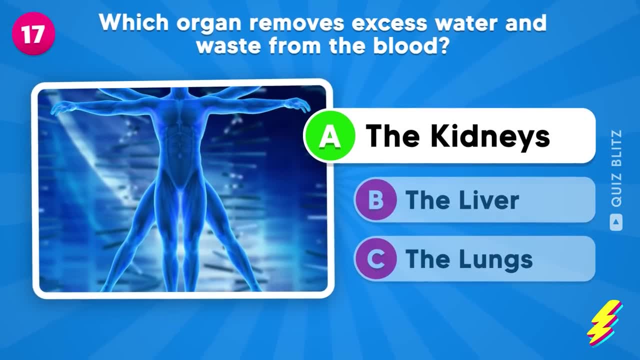 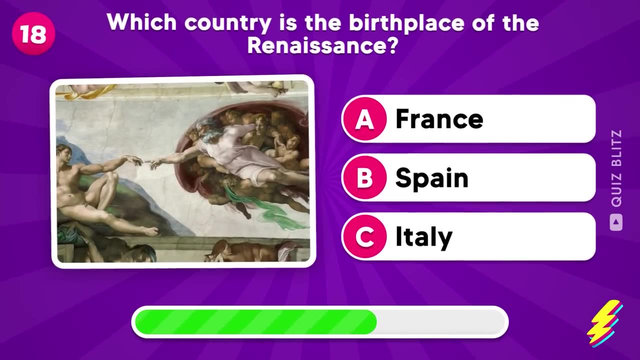 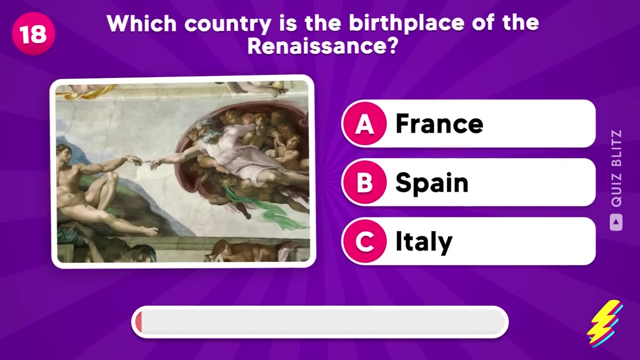 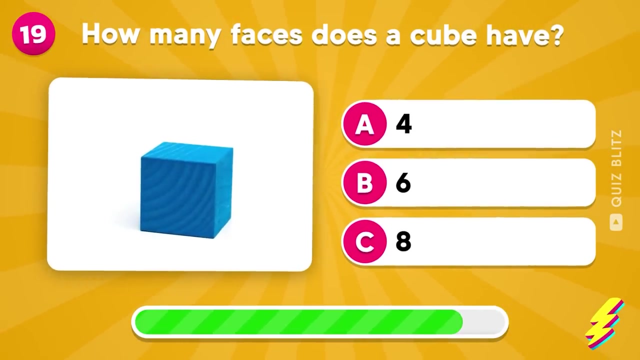 The kidneys, the liver or the lungs, The kidneys, The kidneys. Which country is the birthplace of the Renaissance? France, Spain or Italy? Let's go, Italy, Italy. How many faces does a cube have? 4,, 6, or 8?? 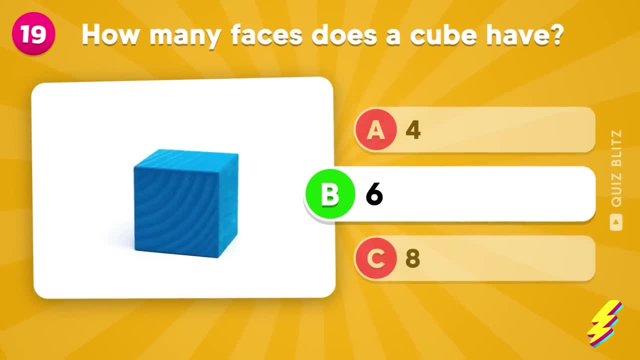 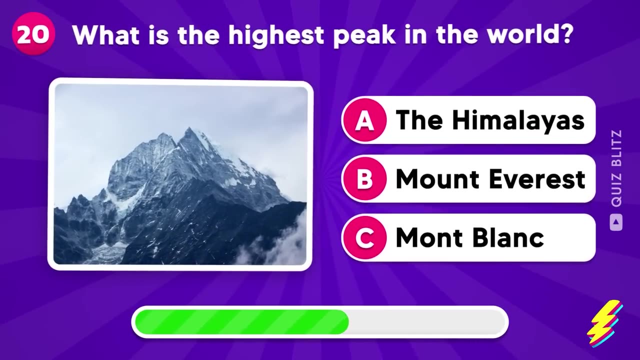 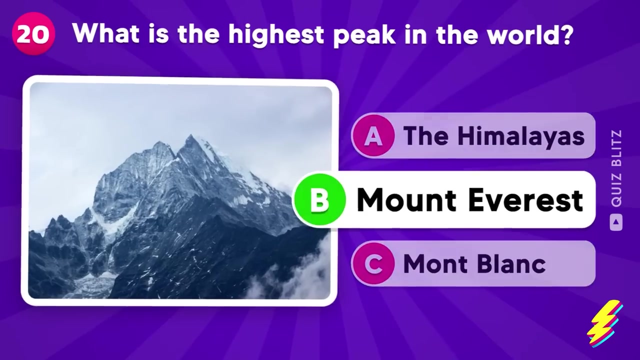 6! What is the highest peak in the world? The Himalayas, Mount Everest or Mont Blanc? The Himalayas, Mount Everest or Mont Blanc? 6! What is the highest peak in the world? The Himalayas, Mount Everest or Mont Blanc? 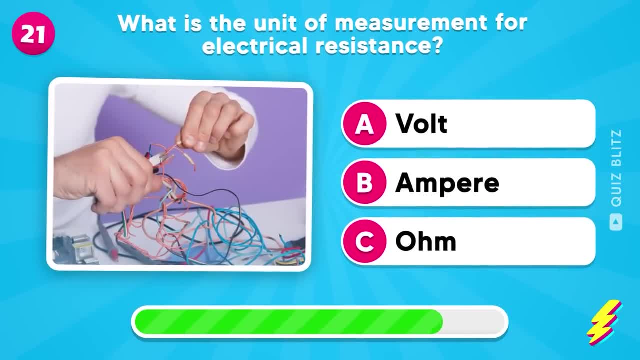 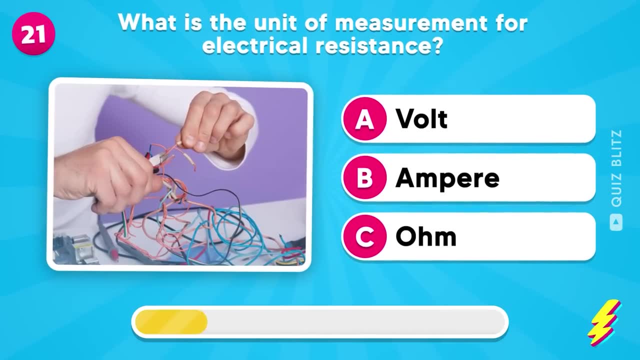 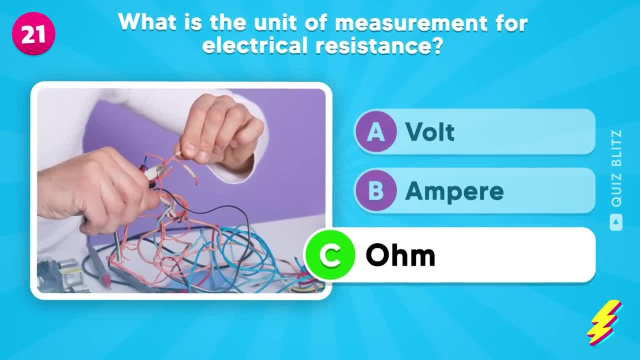 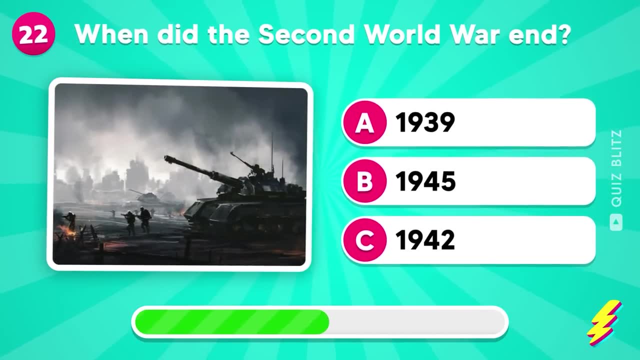 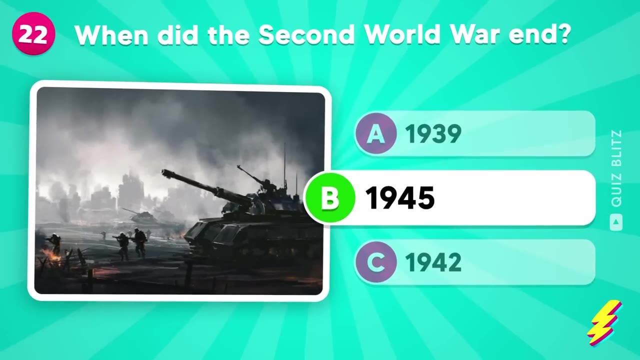 Ohm, When did the Second World War end? 1939, 1945, or 1942? 1939, 1945, or 1942?? Correct, it's 1945!. Correct, it's 1945!. 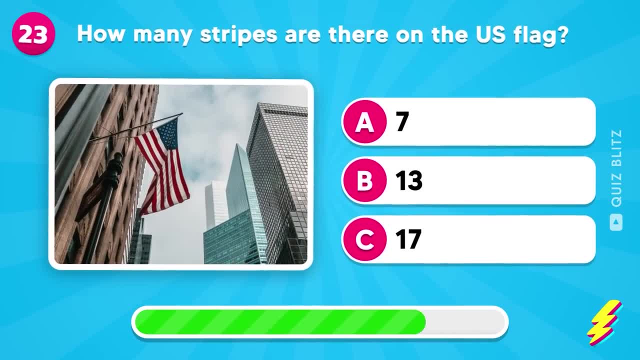 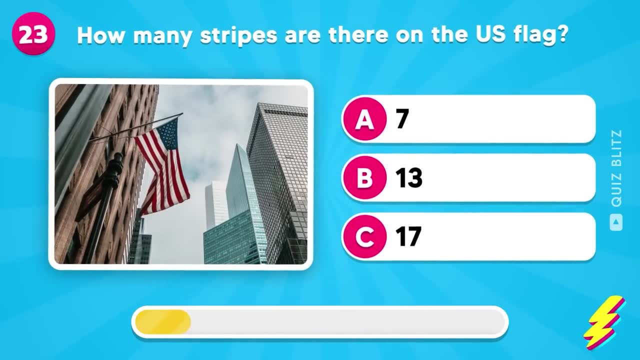 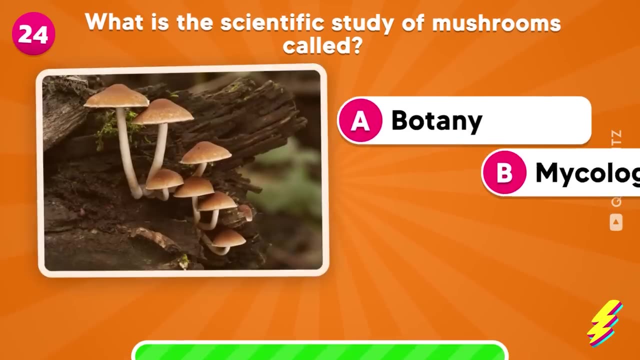 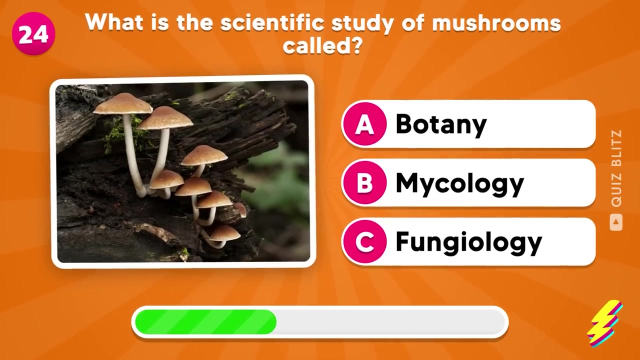 How many stripes are there on the US flag? How many stripes are there on the US flag? There are seven, thirteen or seventeen. There are thirteen. What is the scientific study of mushrooms called Botany, Mycology or Fungiology? 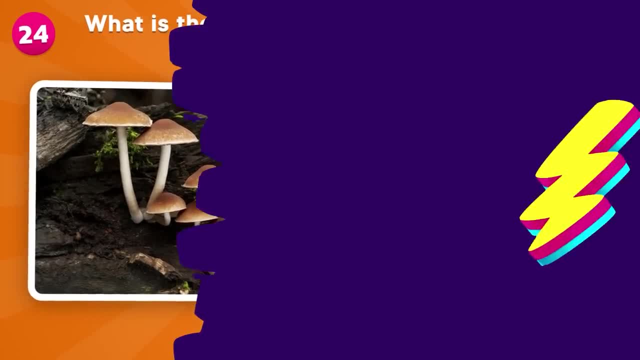 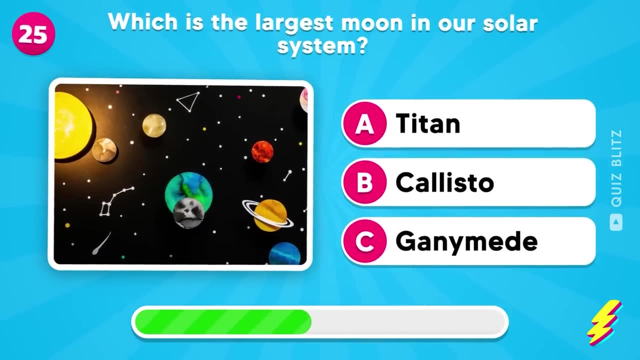 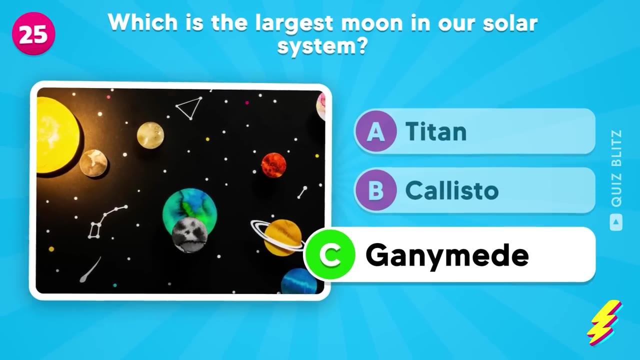 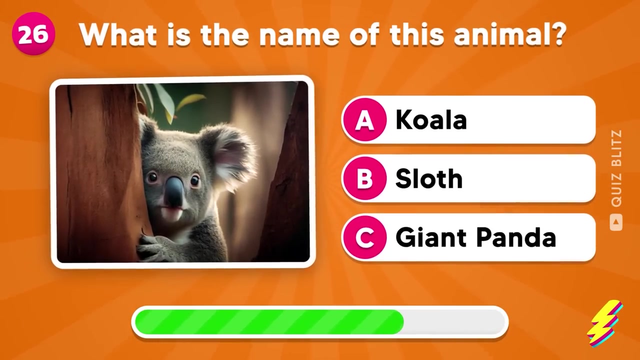 Which is the largest moon in our solar system? Titan, Callisto or Ganymede? It's Ganymede, a satellite of Jupiter. What is the name of this animal? koala sloth or giant panda? What is the name of this animal, koala sloth or giant panda? 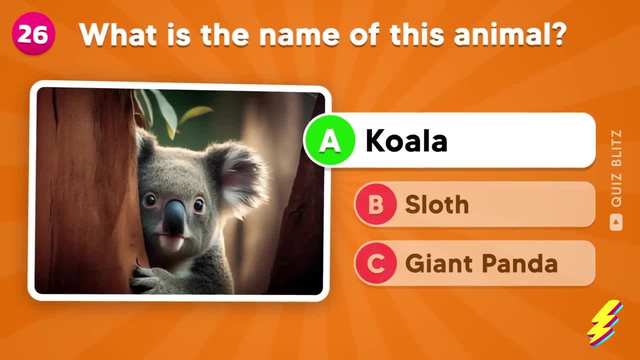 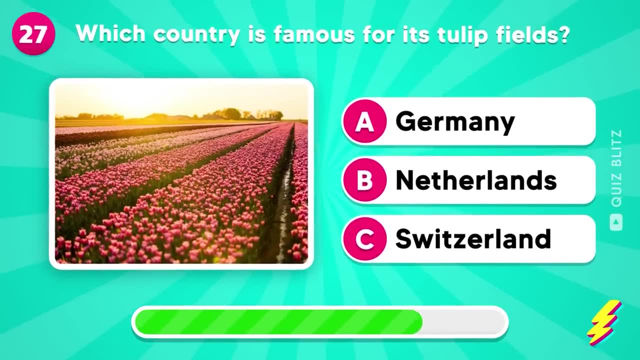 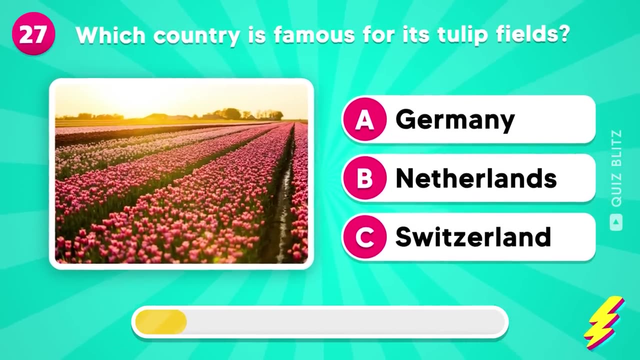 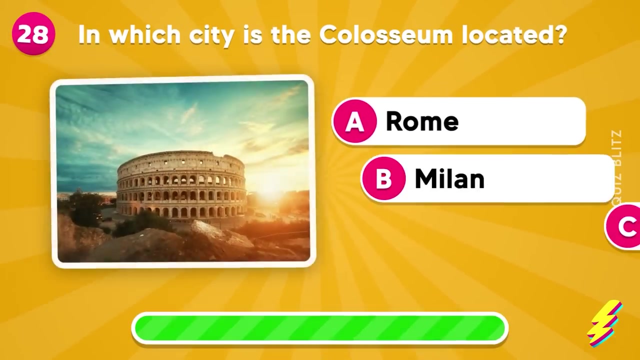 What is the name of this animal? koala, sloth or giant panda Koala? Which country is famous for its tulip fields? Germany, Netherlands or Switzerland? It's the Netherlands. In which city is the Colosseum located? 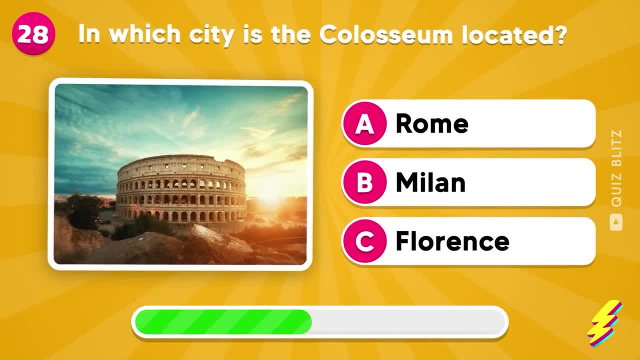 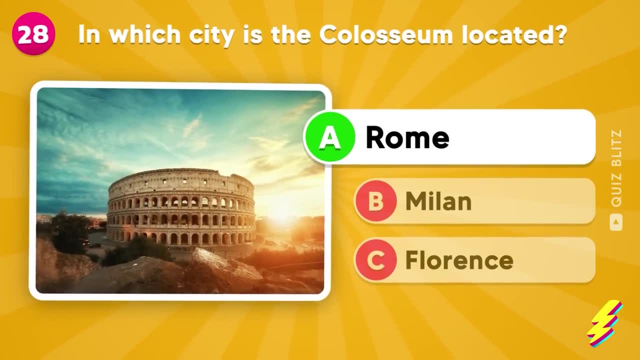 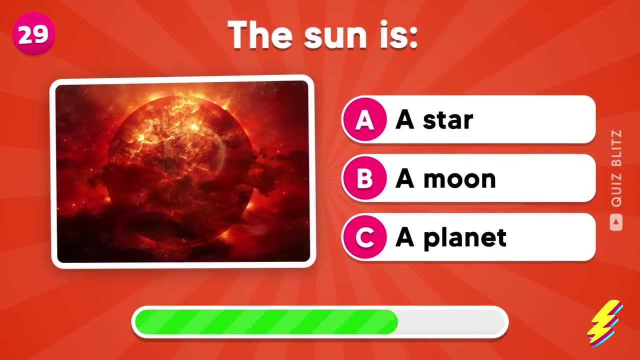 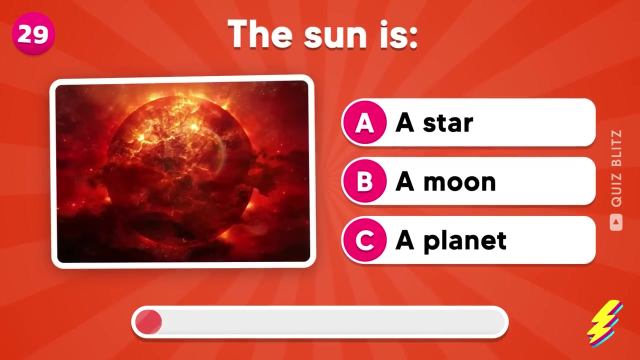 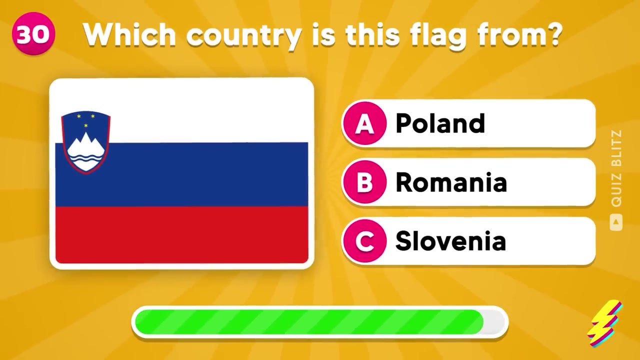 Rome, Milan or Florence? The Colosseum is located in Rome. The sun is a star, a moon, or a planet, A star. Which country is this flag from? Poland? Poland or Poland? Poland, Poland or Poland. 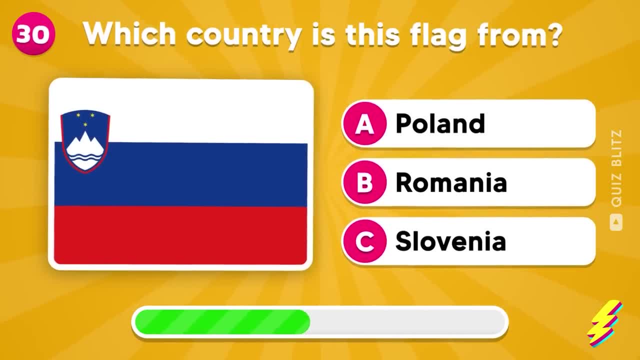 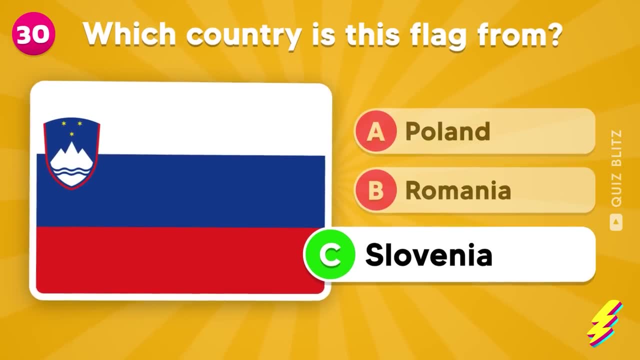 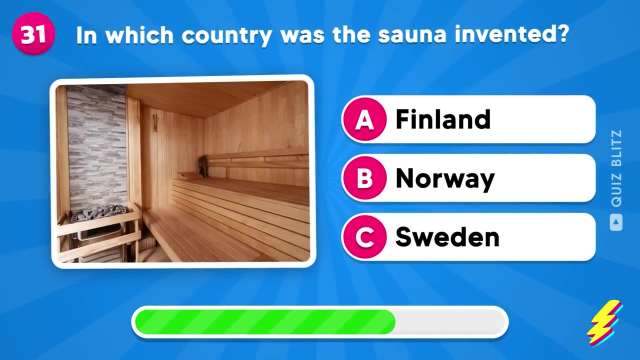 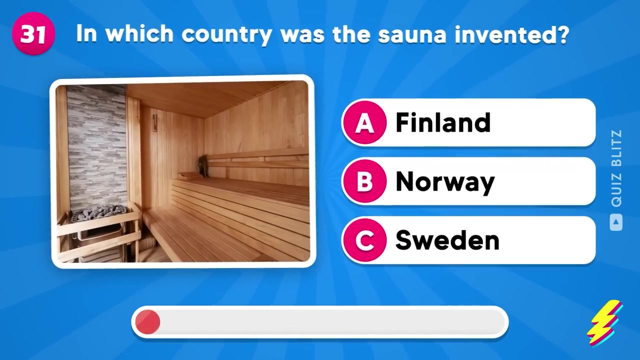 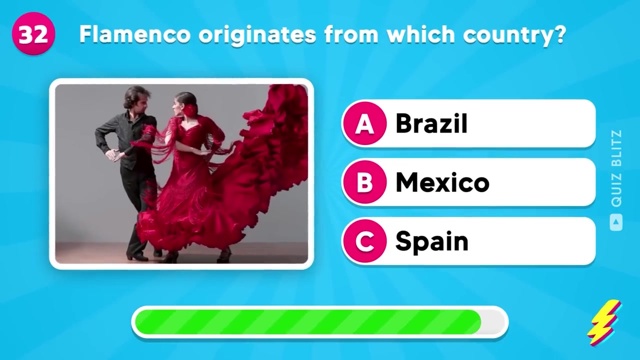 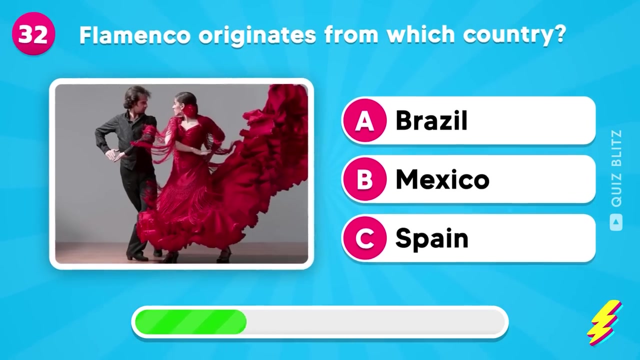 Romania or Slovenia, Slovenia? In which country was the sauna invented? Finland, Norway or Sweden? It was invented in Finland. Flamenco originates from which country? Brazil, Mexico or Spain. Brazil, Mexico or Spain? Yes, it's Spain. 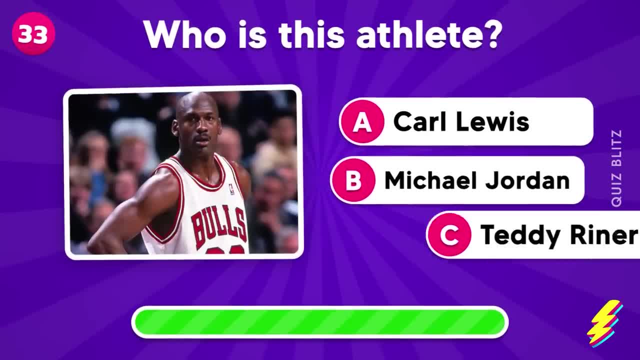 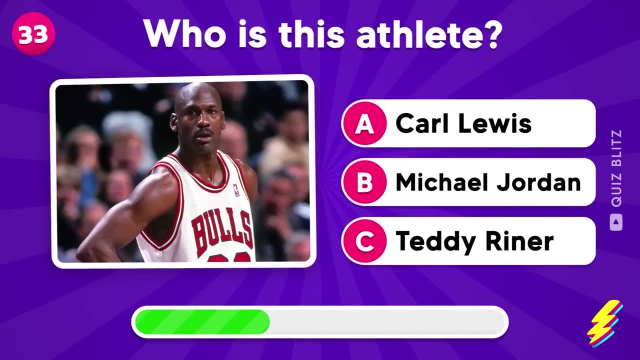 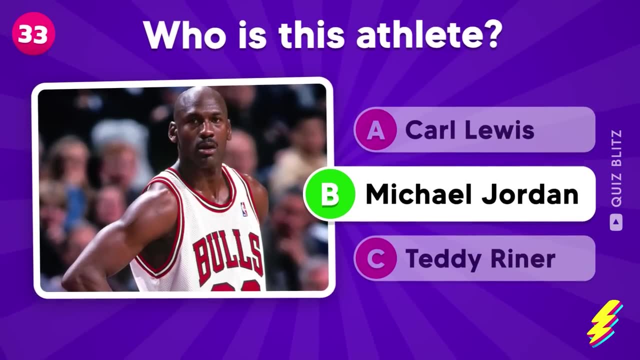 Yes, it's Spain. Who is this athlete? Who is this athlete? Karl Lewis, Michael Jordan or Teddy Riner? Karl Lewis, Michael Jordan or Teddy Riner? Michael Jordan, Michael Jordan? Who is this athlete? What is the capital of Canada? 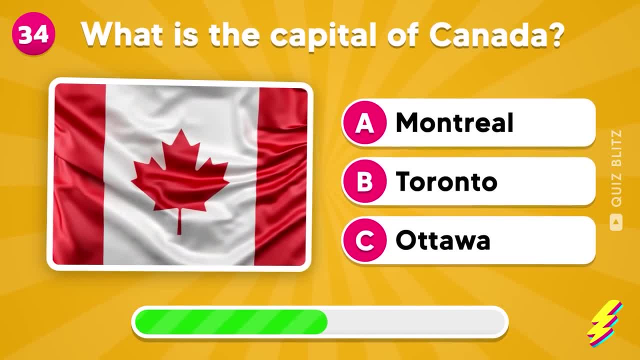 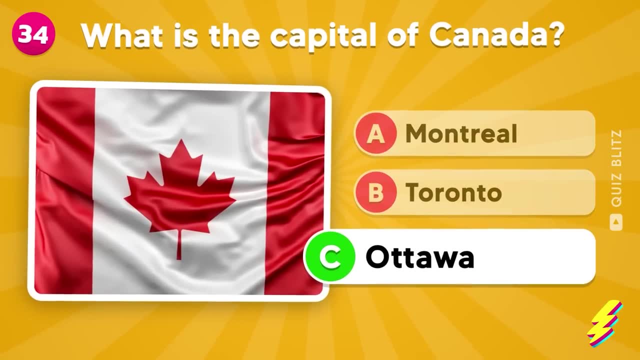 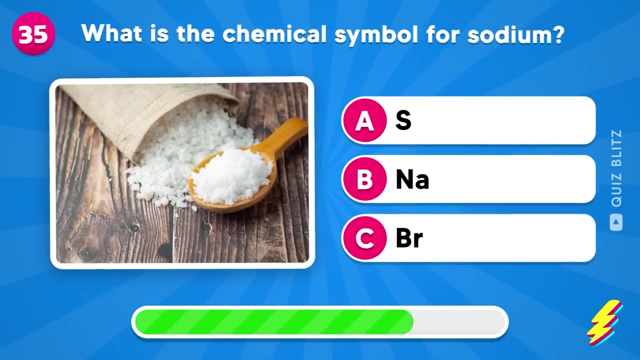 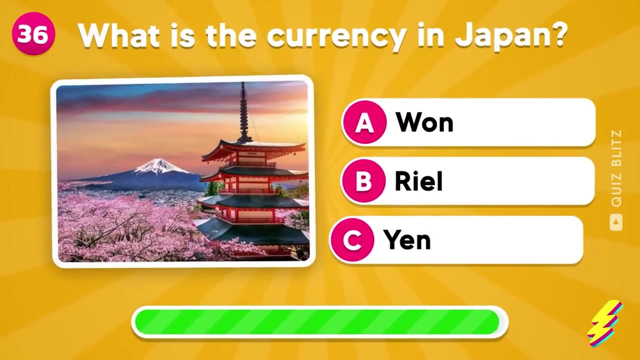 Montreal, Toronto or Ottawa? Bravo, It's Ottawa. What is the chemical symbol for sodium, S, Na or Br? It's Na from Latin Natrium. What is the currency in Japan? 1, Riel or Yen? 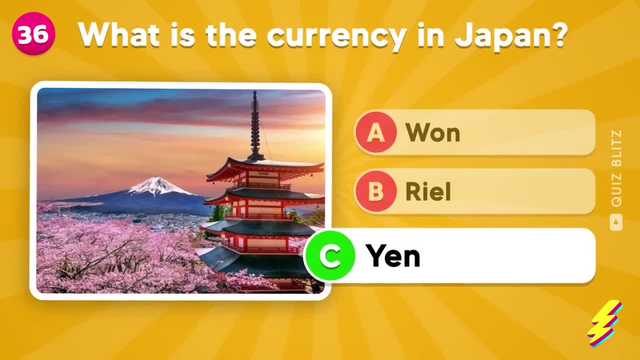 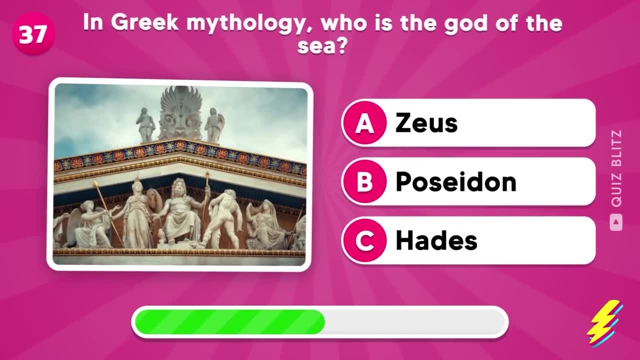 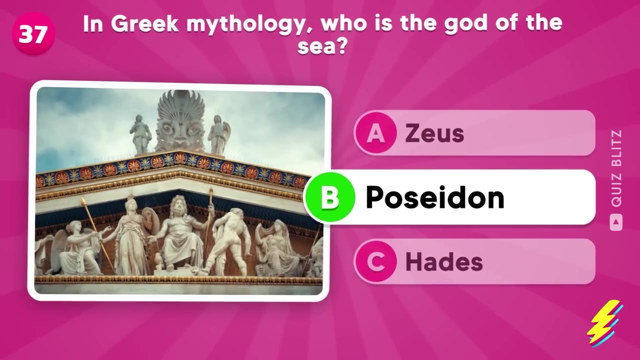 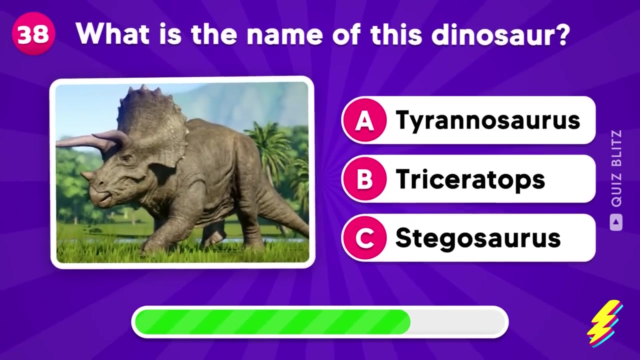 It's Yen In Greek mythology. who is the god of the sea, Zeus, Poseidon or Hades Poseidon? What is the name of this dinosaur? Tyrannosaurus, Triceratops or Stegosaurus? 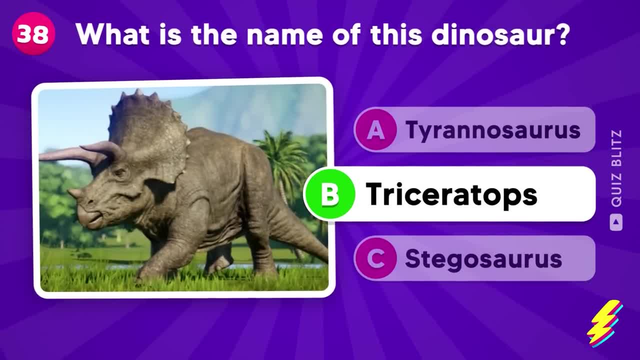 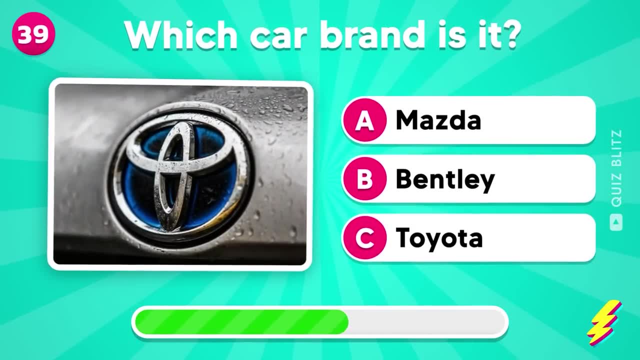 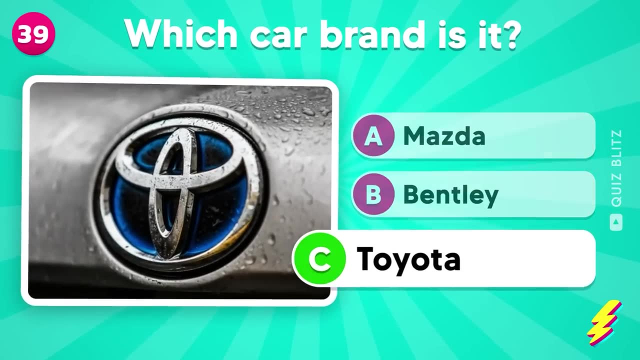 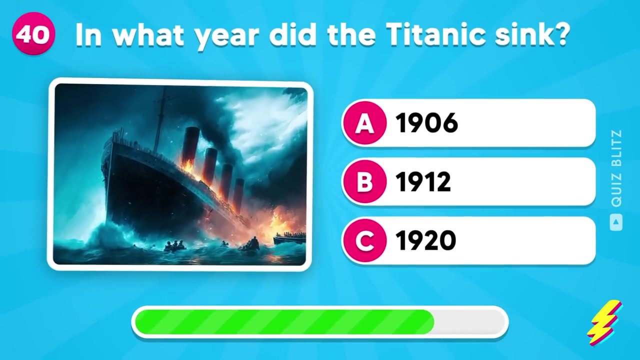 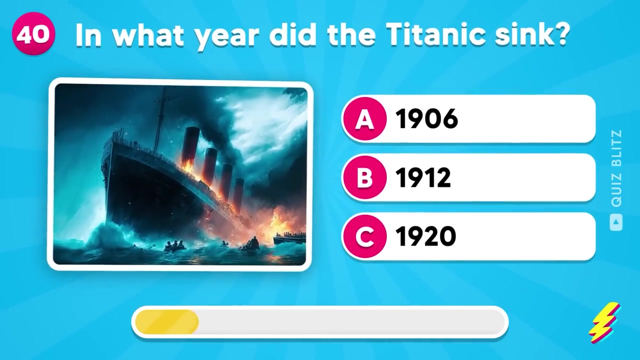 It's a Triceratops. Which car brand is it Mazda, Bentley or Toyota? Toyota. In what year did the Titanic sink? 1906,, 1912, or 1920?? Correct, It's 1912!. 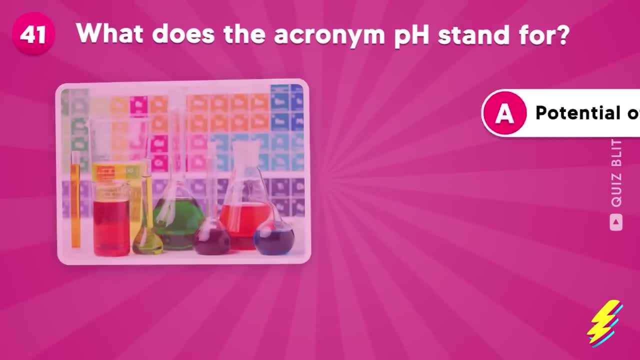 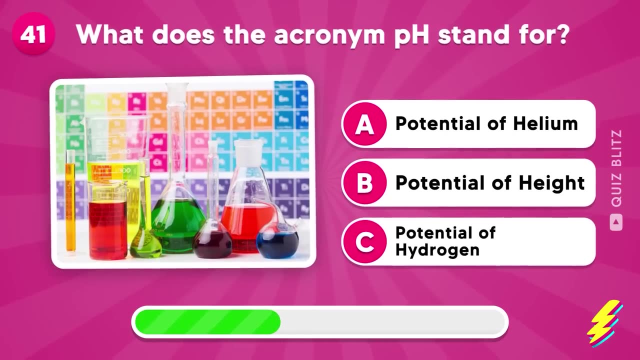 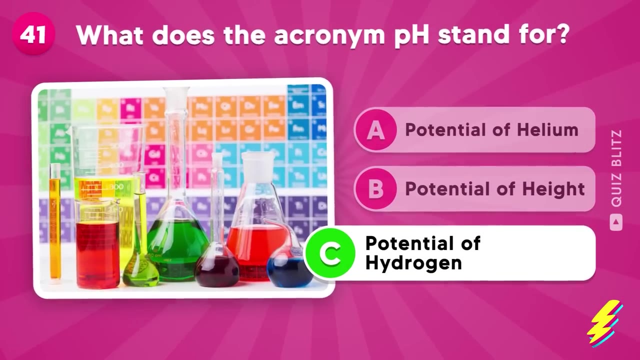 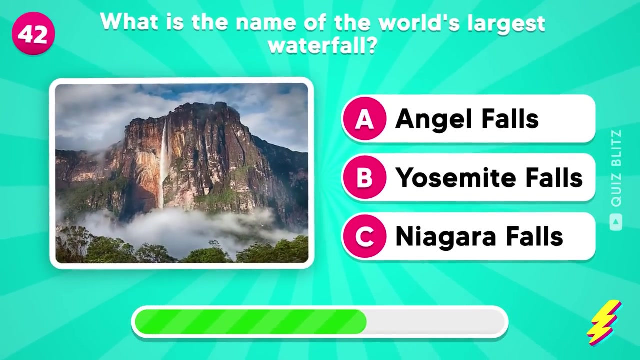 It's 1912!. What does the acronym PH stand for? Potential of Helium, Potential of Height or Potential of Hydrogen? Yes, It's Potential of Hydrogen. What is the name of the world's largest waterfall? Angel Falls, Yosemite Falls or Niagara Falls? 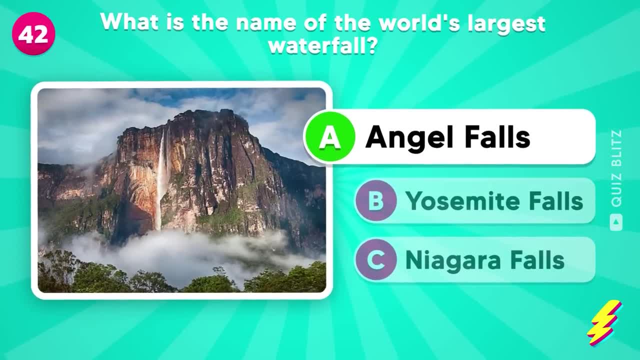 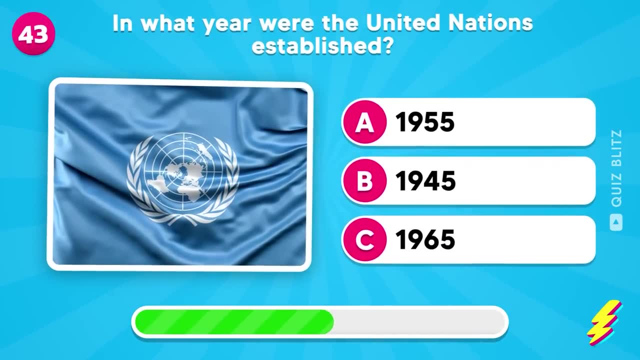 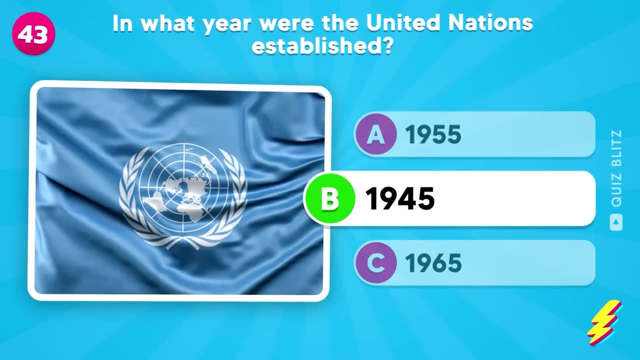 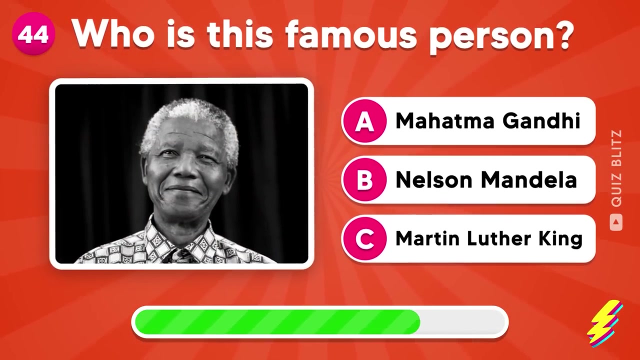 It's Angel Falls in Venezuela. In what year were the United Nations established? 1955, 1945, or 1965?? Bravo, It's 1945!. Who is this famous person? Mahatma Gandhi, Nelson Mandela or Martin Luther King? 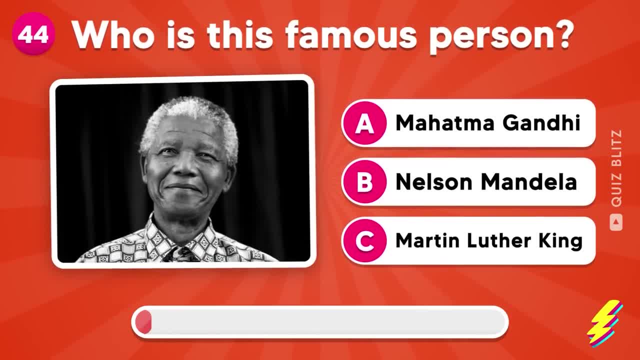 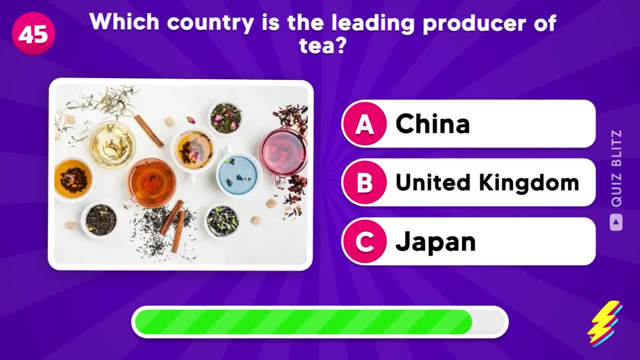 Yes, He was the President of the United Nations. He is a man of philosophy, Nelson Mandela or Martin Luther King? Yes, The American famous American Nelson Mandela a man of philosophy. Which country is the leading producer of tea? China, United Kingdom or Japan? 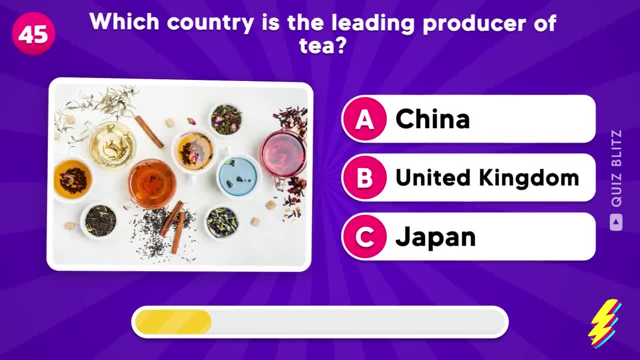 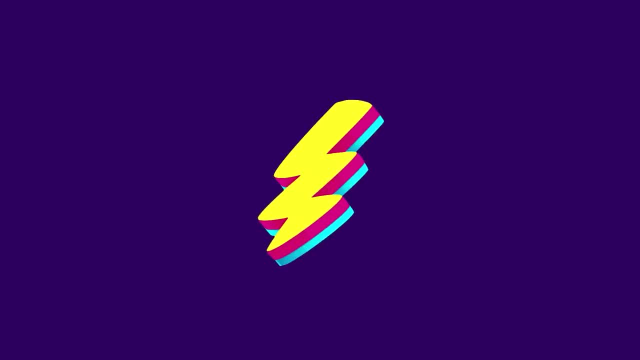